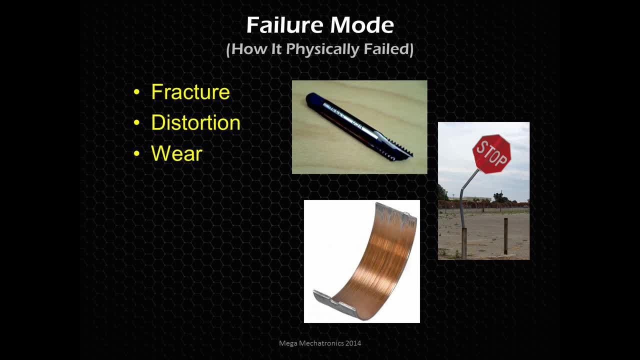 Where, Where can cause lots of problems and lead to catastrophic failures or even fractures. So this is an engine, a bearing that was probably from- yeah, it's from- an engine. when those like a rod bearing blows out, then you start heating up your crankshaft and you're you start you can even break your crankshaft from the excessive heat and that's ruining your heat treat and fatigue, perfect protection, and then you overstress it and it breaks. So where can lead to failures and inefficiencies and catastrophic failures. 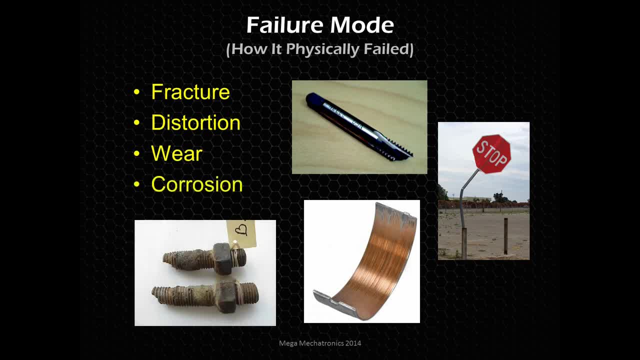 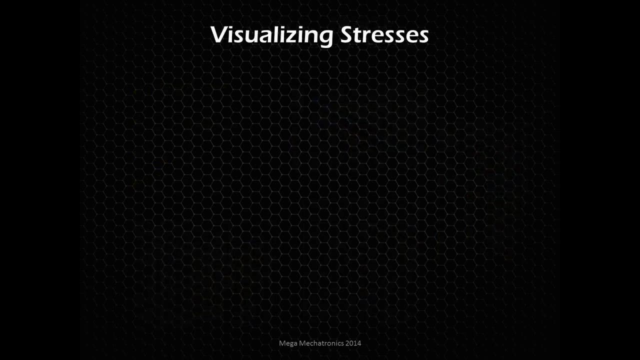 And corrosion. Corrosion can definitely lead to excessive wear, distortions and, most likely, fracture. So how can we visualize stresses- And I'm bringing this up because we need to learn where to expect a failure in a part. So if we understand the stresses a little bit more and stress concentrators, things like that, we can. we. 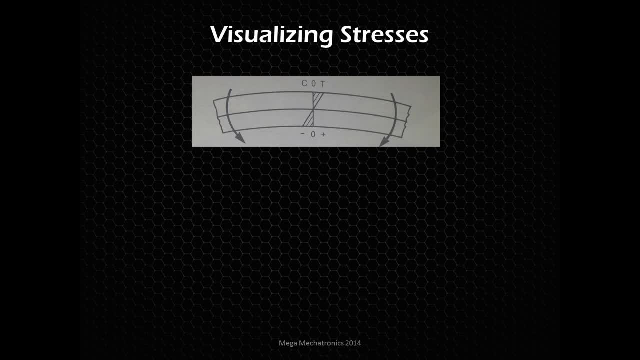 can get a better idea of what was expected. so, for example, let's take a look at this picture and it might look confusing at first, and I don't blame you. what this is is the section of a part, so physically that how that part looks, plus a graph that's integrated into that, a physical layout of 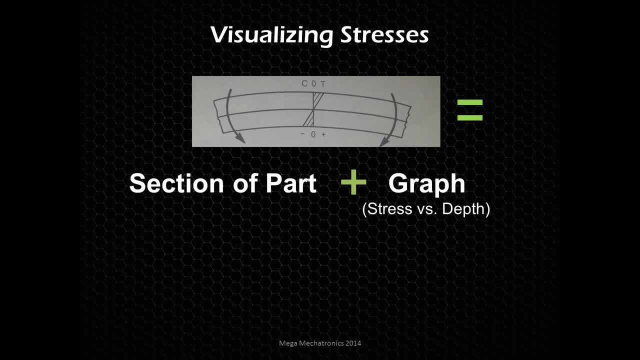 the, the graph within the physical layout. so the graph actually corresponds the physical shape of that part. so you can see there's a C, a zero and a T and that's representing a compressive stress and negative stress, and then going to the right is a tensile stress and then for our other scale, 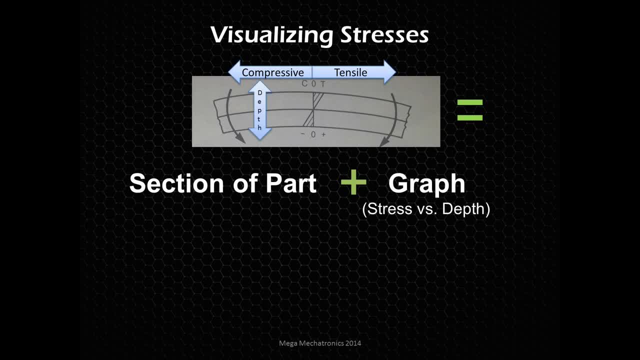 of this graph. we're going to take a look at this graph and then we're going to take a look at this graph. we have the depth, so you see, the top edge of the part is actually that top edge, that there's a line in the middle. that's actually the middle of the part, and then go on the bottom, the bottom side. 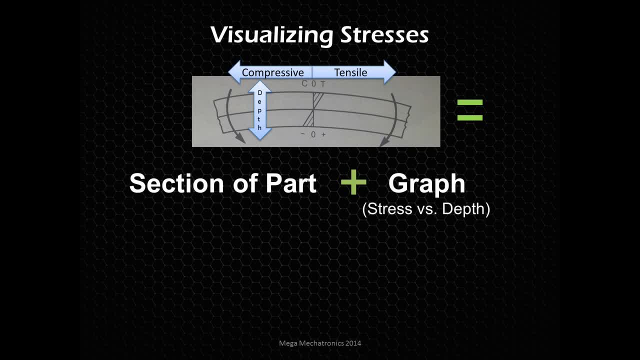 so if we analyze this graph, what you're looking at on the top side is a tensile stress, and since that line is on an angle that shade it's- it's cross hatched, you can see the maximum tensile stress that this part is seeing happens to be at the very surface of the part, and then we move into the middle and you see. 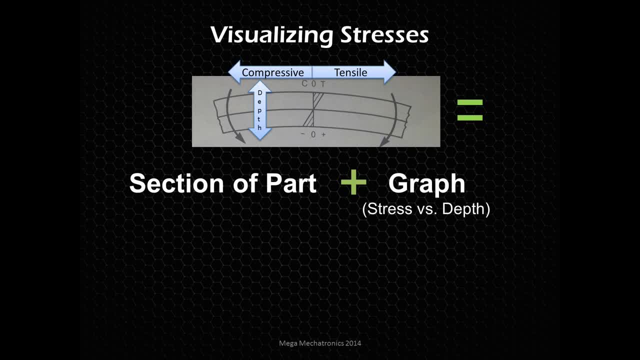 there's no stresses there. you can almost think of that as like the pivot point and this- this is a very symmetrical example as well, but we're just trying to get the idea across. so we have our tensile up there and then we're moving to the bottom side and what you're seeing obviously at 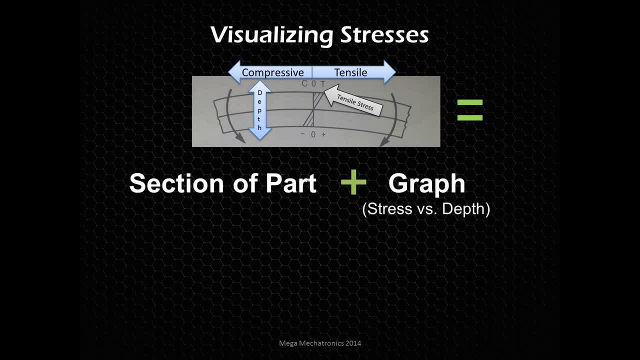 the very bottom edge is the maximum compressive stress just happens to be at the very surface and that's typically how parts react to stresses, where the surfaces are being the the max stress. and in our video example you can again see how i'm bending that piece of paper and it's going to pull apart at 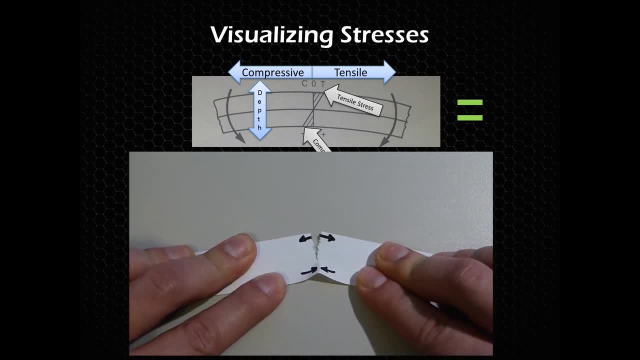 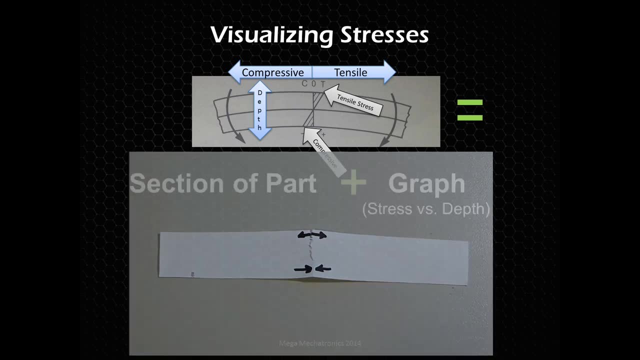 the top because it's under tensile, and then you see it buckling at the bottom because that paper is trying to remove it and it's going to pull apart at the bottom because it's under tensile and to come together, but it will buckle up. 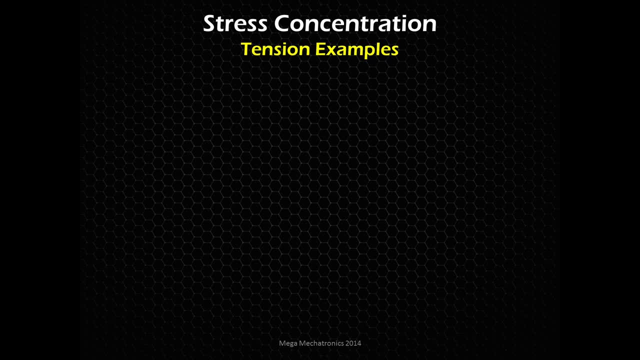 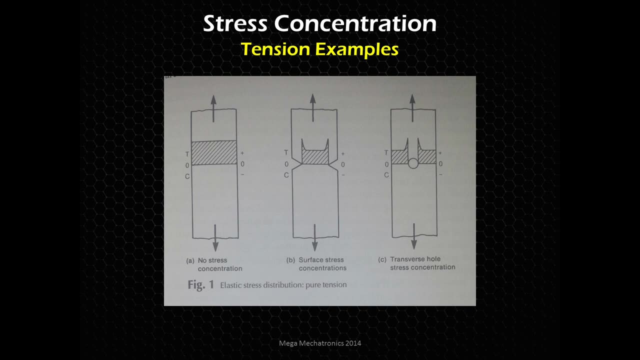 So, moving into stress concentration, let's look at some tension examples. So on the very left, A is a part being pulled apart, just like a tensile stress that we talked about. So you see there is no stress concentration because that line, that crosshatch line, is straight across from edge to the 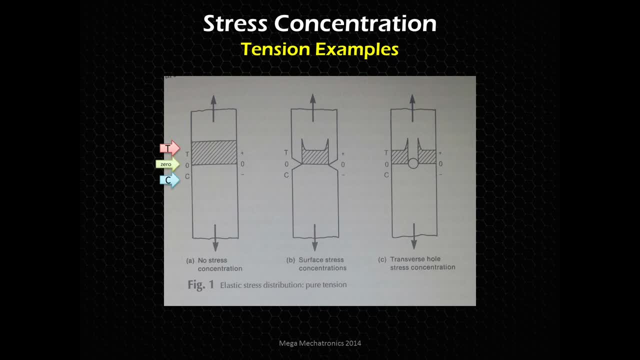 center to the middle And you see there's a zero point. it's under tension and here's the center and it's equal across the top. So, moving to the middle example, we see a couple notches cut into the sides, the 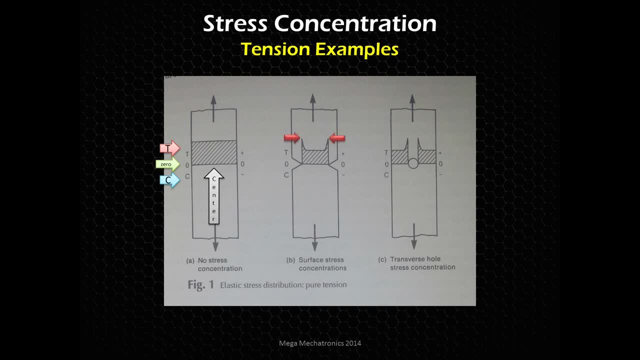 edges and we see there are stress concentrations here. You see these spikes right at the very edge inside of those notches And then we have a hole that's drilled through this part And again these are under pure tension. these are being pulled apart. 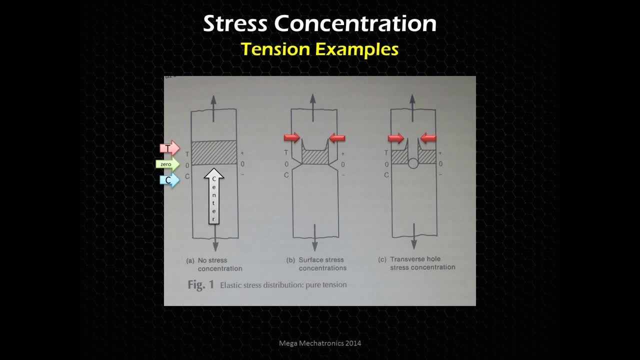 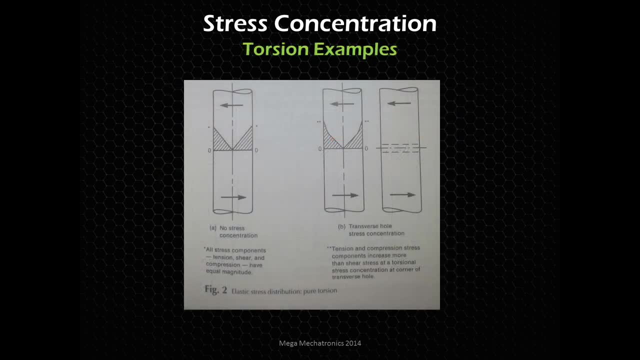 And you see there's stress concentrations at the very edges of that hole, Those spikes. And now let's look at a torsion. This is where we're twisting this rod, or this part, right here. So again on the left, we see there's no stress concentrations. 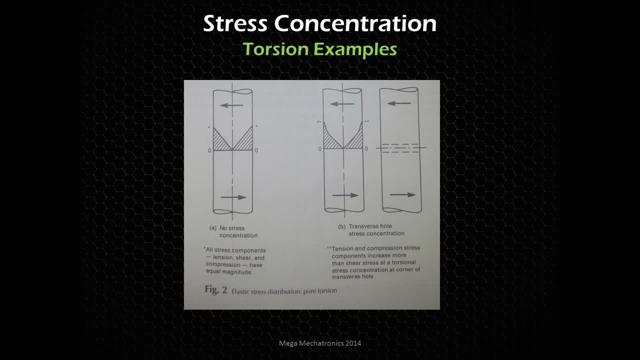 And because we are twisting it, you see there's no stress in the middle because, again, that's almost like a pivot point, And then the max stress is on the very surface, and that's just how materials react under a torsion. 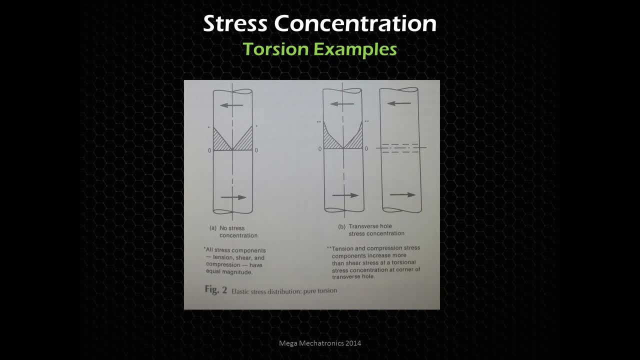 But then on the right we have a hole that's drilled through. So you see that the phantom line there showing a hole that's drilled through And again this part's being twisted, It's under a torsion and you see, there's stress concentrators. 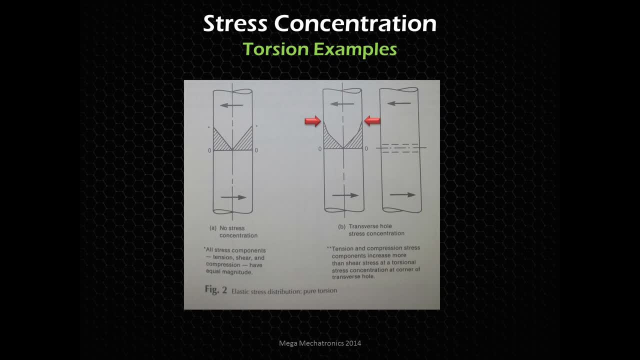 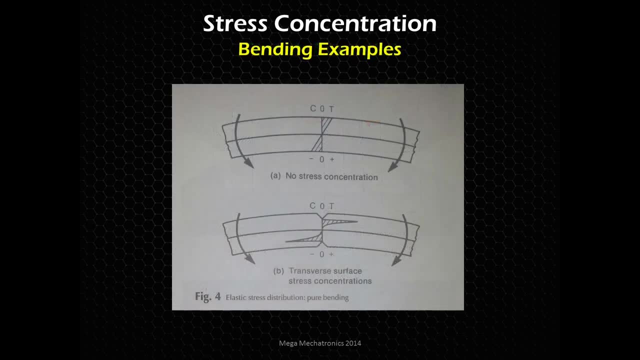 under tension side, on the very edge, outer edge, where the drilled hole is. And going back to our bending example, there's something a little different here Because, remember, with this bending example we're having both tension and compression And you see how those notches in the part create the 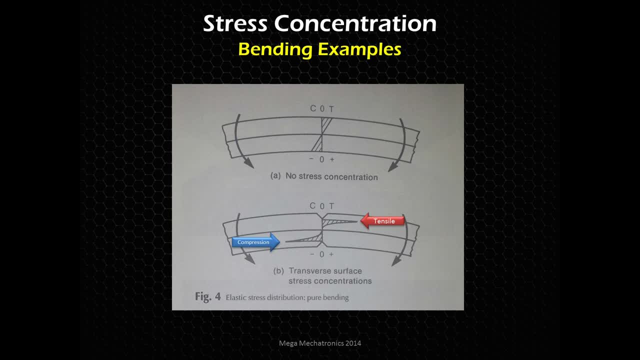 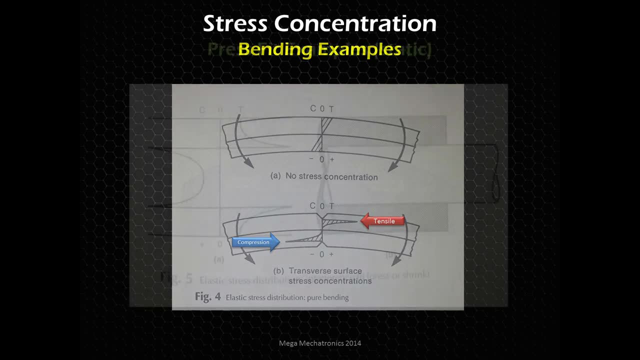 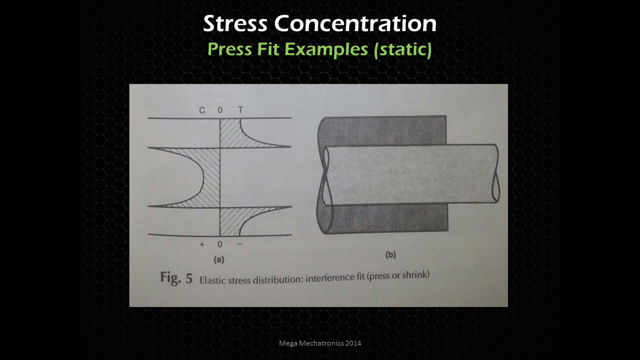 tension and spikes in tension on the top side and there's a big spike in compression on the bottom side. And again, this is pure bending And here's like a press fit example, in a static It's not being bent or anything. This part there's a. 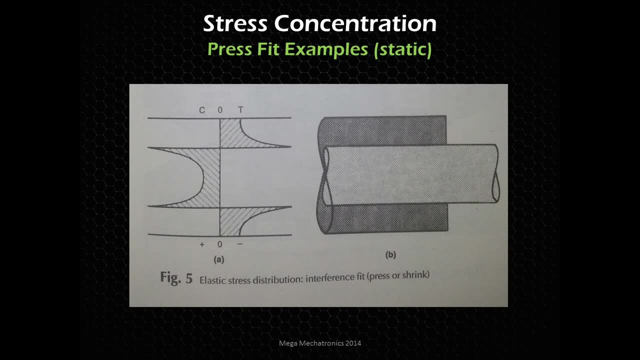 rod being press fit into a tube. So you see the tube's inside surface is under tension, right at the inside surface, And that makes sense because that rod is trying to push, stretch that tube And then to balance that out. the rod is under compression stress because that tube is trying to squeeze. 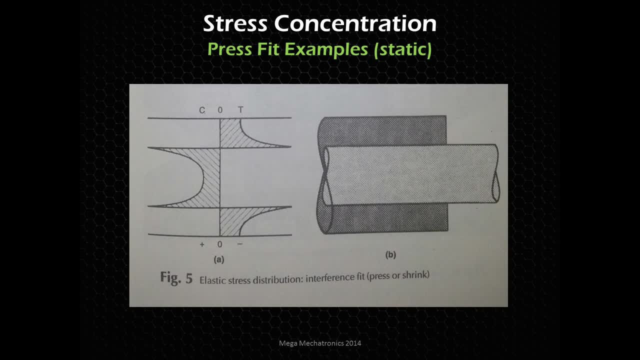 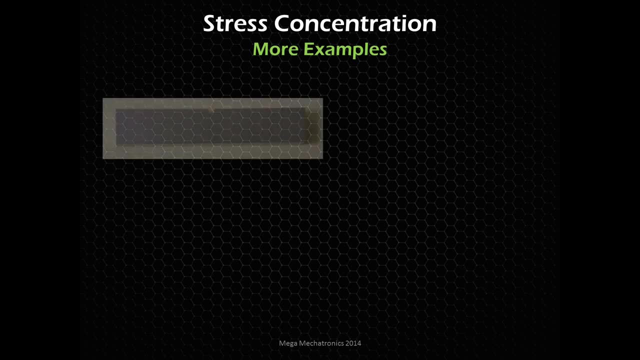 that rod together And that max stress on the rod is at the very surface under compression. So some more examples. Here's our Sharpie test. And remember that notch. That's put there on purpose so that gives the scientists and engineers a consistent place. 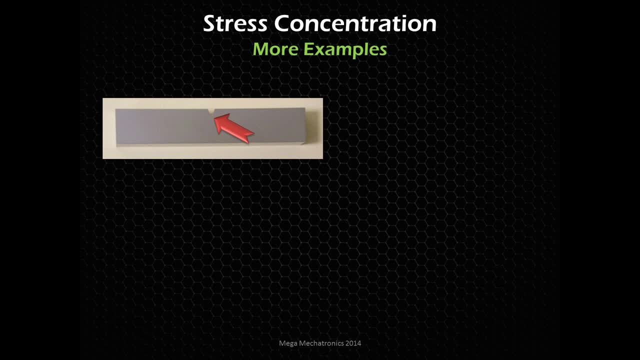 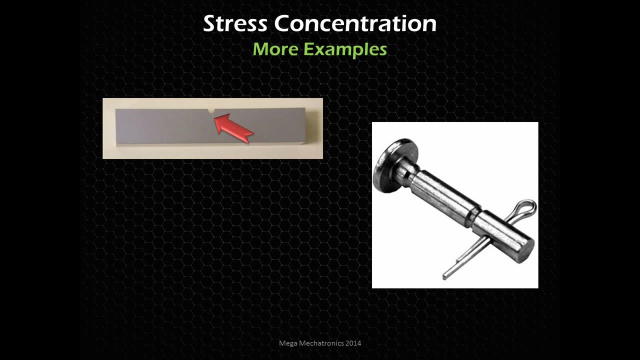 where that part is going to fail, And that leads to more consistent test results. And let's look at this shear pin. This is like a snow blower where you can control how the part fails And the failure mode, So you know if something. 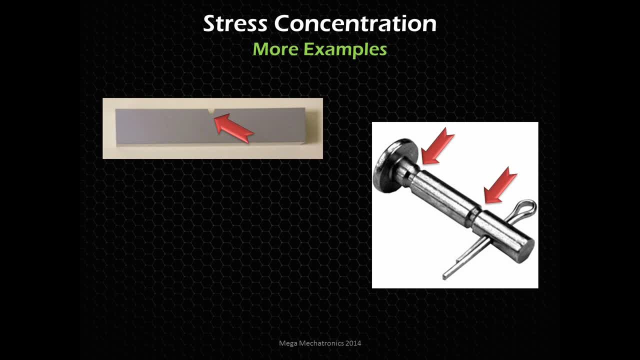 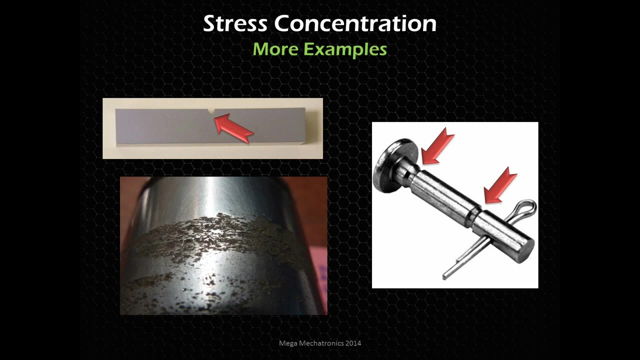 gets jammed in there at a certain force, this pin will break. And it will break at these points and give us a predictable and, most likely, safe way of breaking. And over here we have corrosion pitting And this creates stress concentrations. You see, at a microscopic level. 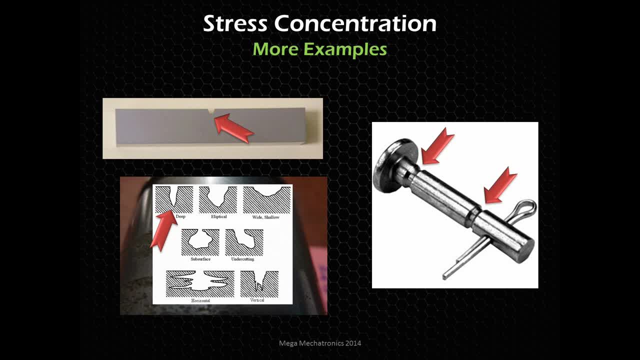 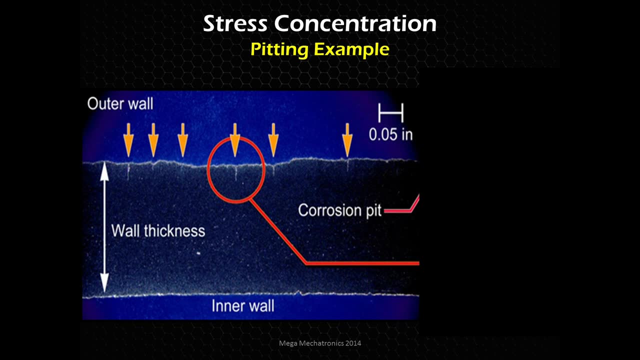 and a couple pits here have some very deep and sharp points of stress concentrations. But all of these are examples of a stress concentration And looking at another example of pitting, we see like a shaft here with corrosion and then these pits And if we zoom in, 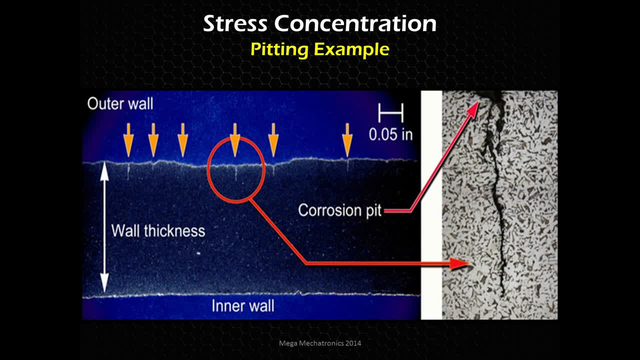 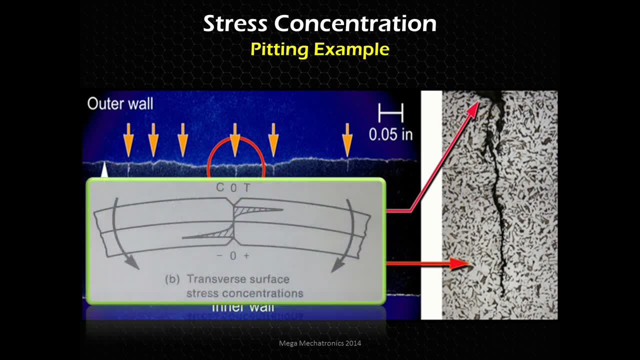 you can see, there's the pit at the top, and then that led to a crack that started at the bottom of the pit, Because those pits are acting like stress concentrations, Again going back to this pure bending. so you see that notch is synonymous with that. 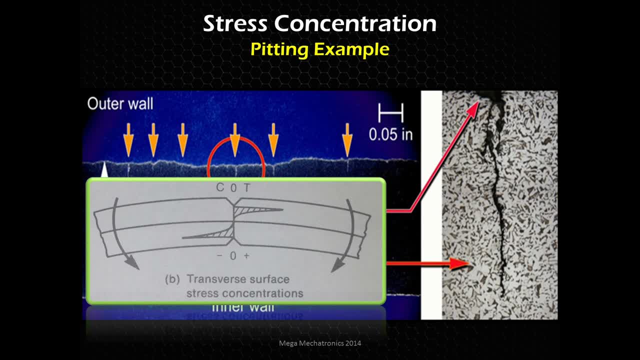 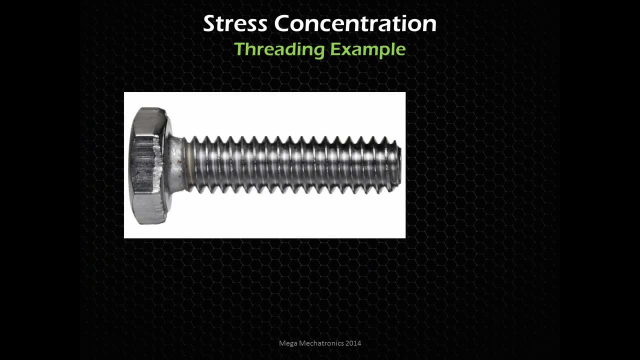 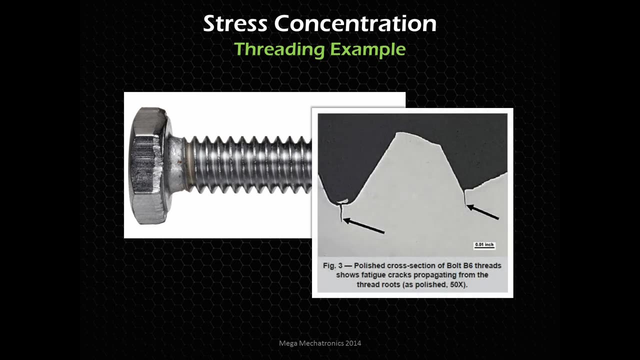 pit. So it's creating a stress concentration there of excessive stress And even threads. You can see threads are filled with stress concentrations Because a bolt's going to fail at the root or the bottom of the thread. That's where likely your failures are going to come from. 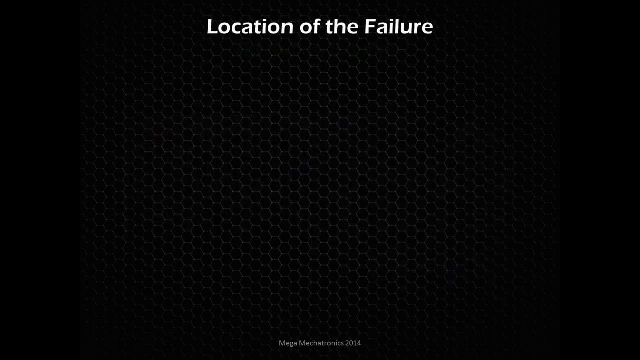 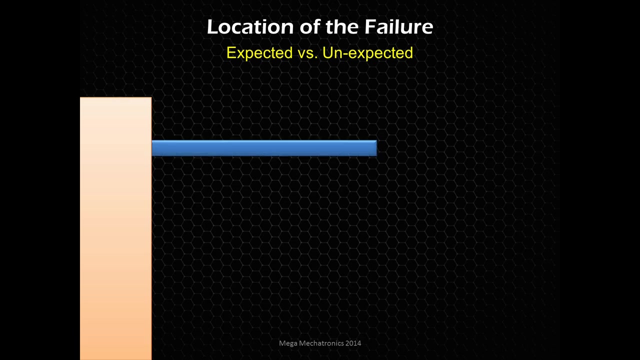 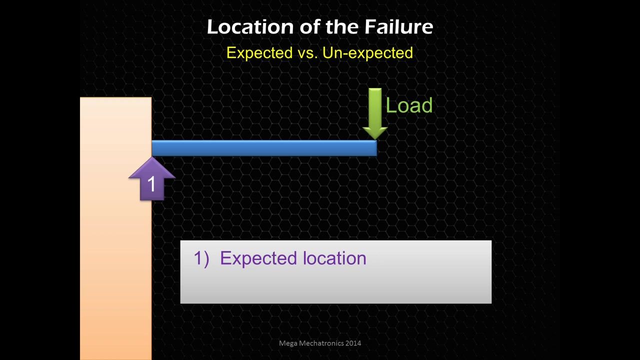 So the location of the failure is very important. So let's say we have a fixed structure with a bar that's attached to it And we apply a load to this At this point, where it attaches to the fixed structure. that's where we would expect it to fail. 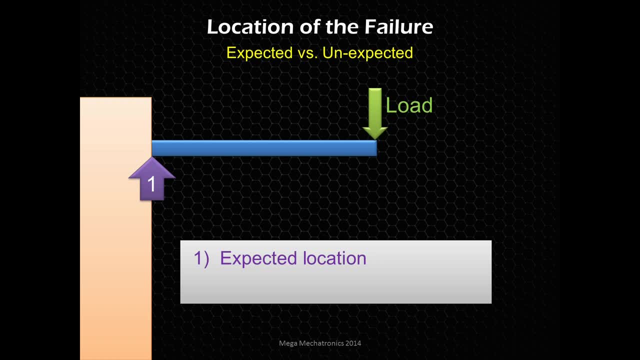 Because that's where we would expect it to fail, Because that's where the max stress theoretically should be on a type of load like this with a bar. However, if, let's say, the bar fails at this point, that's unexpected. We didn't expect. 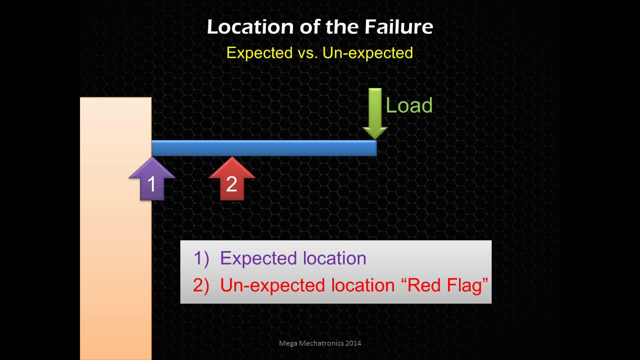 it to fail there. We expected it to fail at one. So what this is is a red flag for you. to just look a little deeper: Was it corrosion? Was there damage there? Was there a scratch, A gouge? What happened? Why did it fail right there? 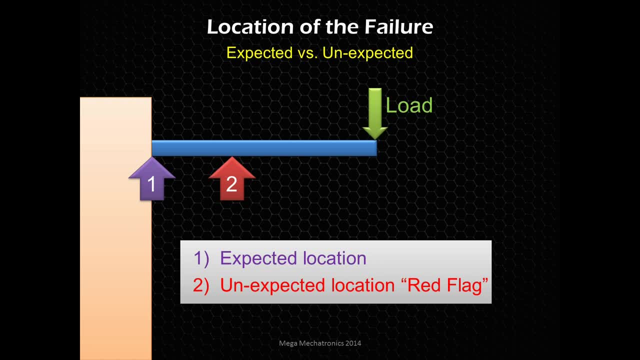 Did the paint chip off and cause corrosion And pitting And these things. So that's something to consider. And while I was touching on those stress concentrations and diagrams of how parts are stressed, because you want, you should have that knowledge of where things are expected to fail, versus unexpected. 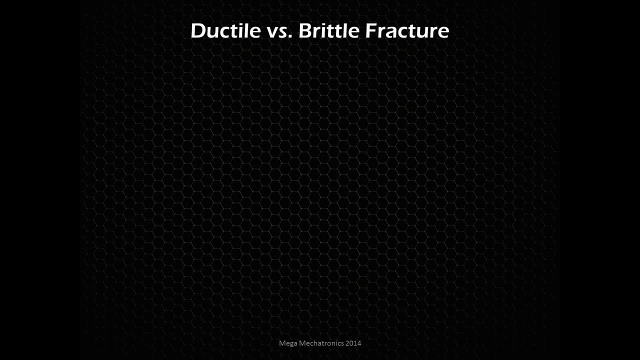 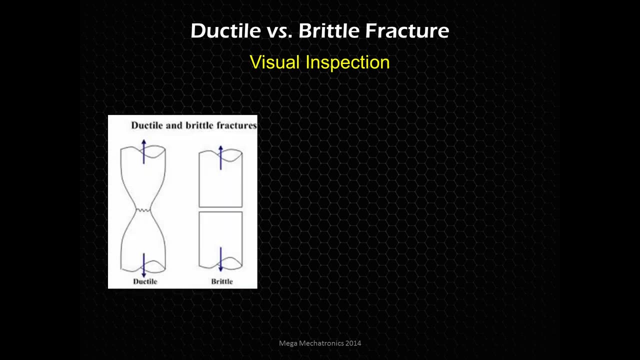 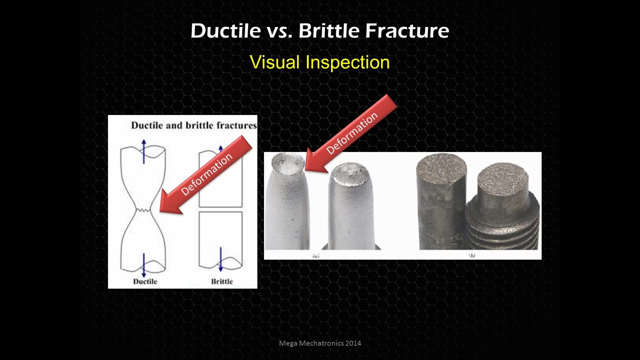 So let's get back into ductile and brittle fractures, And this can be easily done by visually inspecting the part. So again we have deformation Where the parts move, And then even brittle failures, And those are indicators of possibly you're using the wrong material. 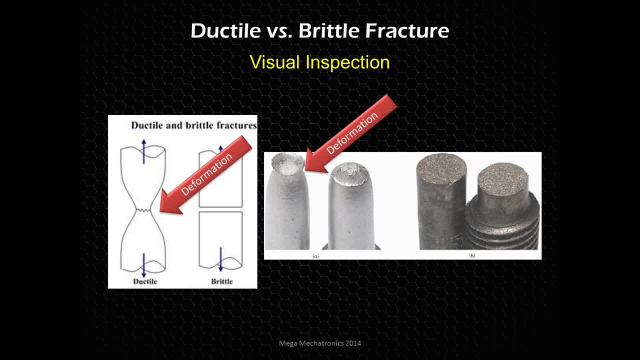 Or something's wrong, Or maybe you need to make some changes. Maybe the bolt you're using is strong, but it's too brittle And it's breaking and falling apart. Where you could put in a little, maybe a softer bolt, that would bend. 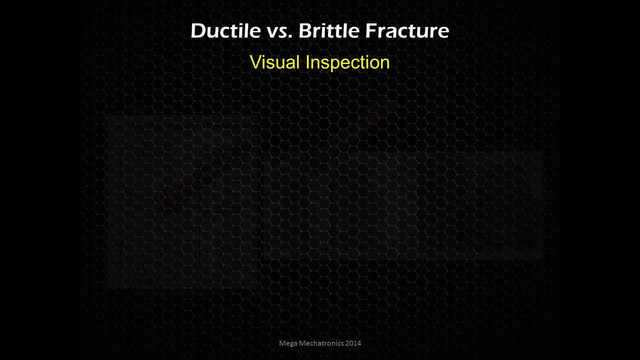 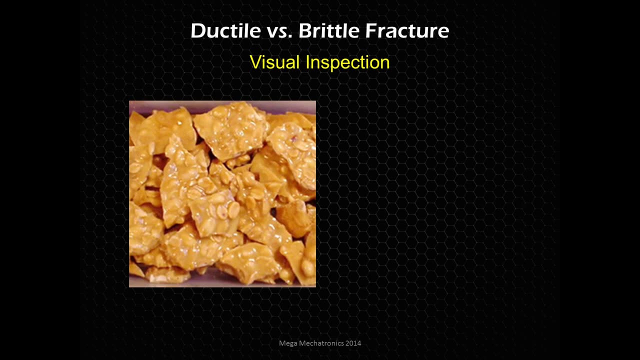 instead of completely failing. So touching on the brittle fractures a little deeper. Let's say you had a bunch of time on your hands And someone said, hey, can you put this pan of peanut brittle back together? You can do it, Because this peanut brittle is extremely hard. 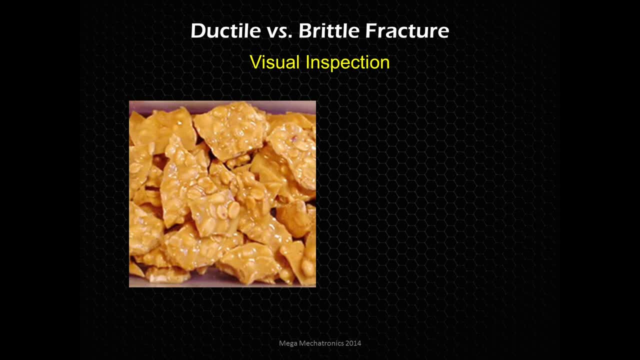 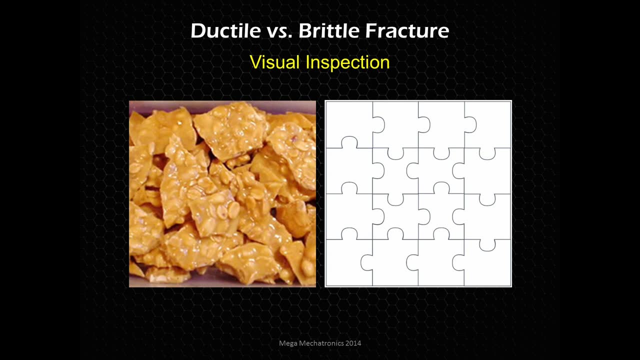 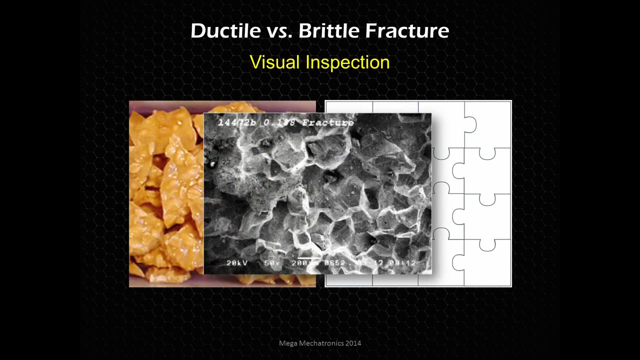 and very brittle And you can actually put the peanut brittle back together like a puzzle, Because those little nodules on these puzzle pieces are intact and will fit back together. And then, looking at like a metal, a brittle metal, you can see there's thousands of these little nodules that stick. 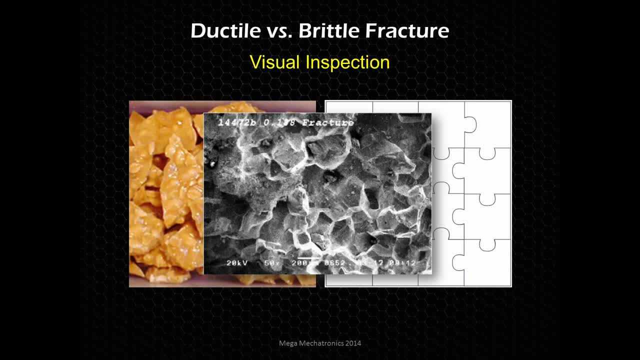 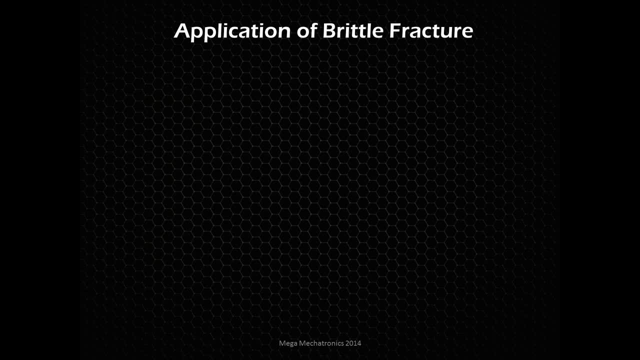 out, But they are stable and the pieces can go back together And these crystals will line up again. So to sort of make that a little more clear, let's look at an application of a brittle fracture and how we can use that brittle fracture. 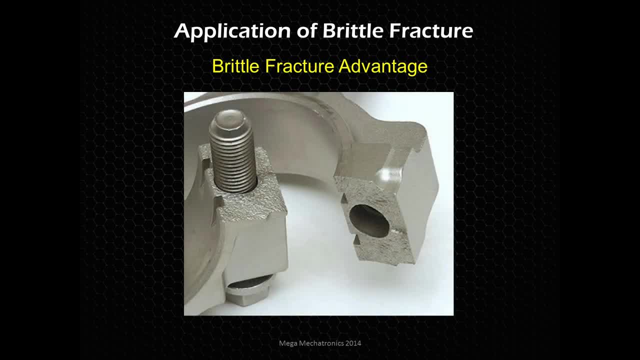 to our advantage is with automotive rod end caps, And these even come from the factory High performance. These are cracked cap rods, So they'll build this rod end and they'll put it in a special fixture and just crack it off. So the advantage is a very 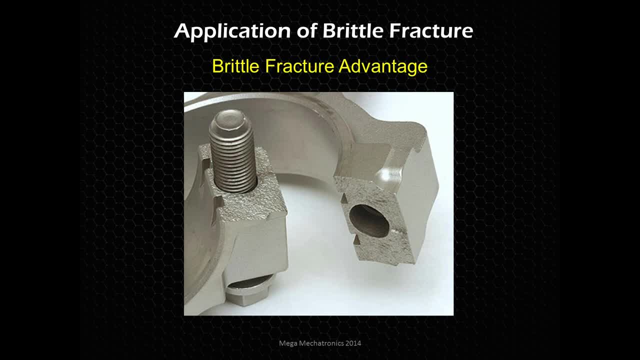 stable mating surface. So when you put these back together and when the engine's on their load and it's vibrating and things like that, these caps are going to be perfectly aligned and nothing's going to change that. If you torque it down to the right spec, it's going to be. 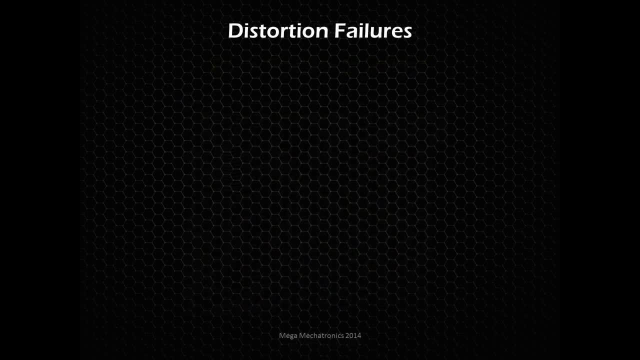 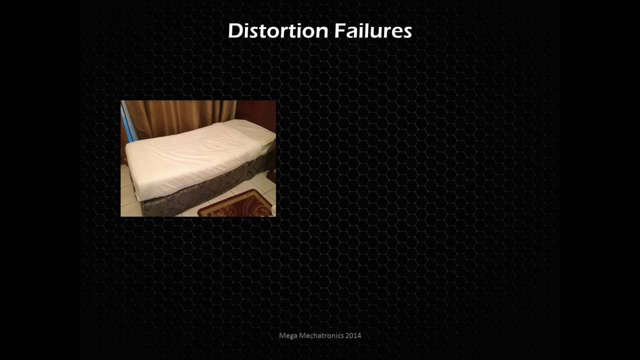 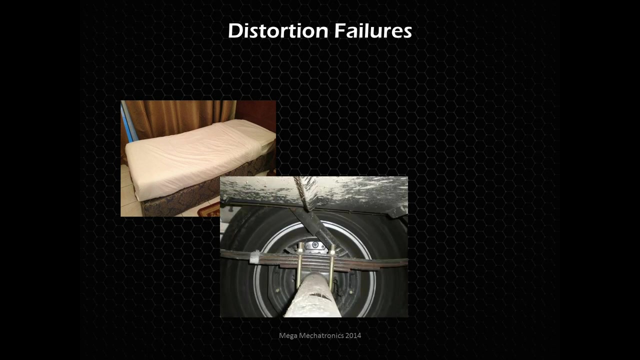 very stable, And here's some examples of distortion failures: Old hotel beds: the bed springs are distorted, They lost their load, They lost their height, They are being bent down more easily and they're sagging. And then here's a sagging leaf spring on a vehicle that. 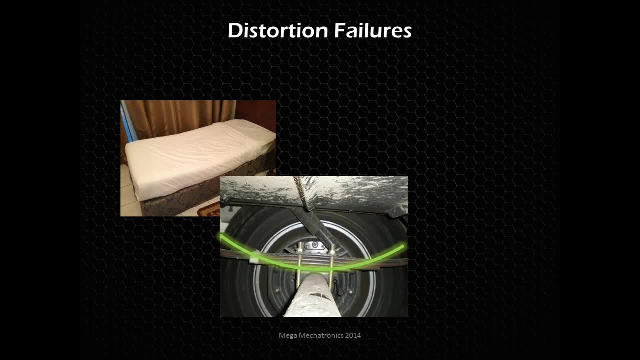 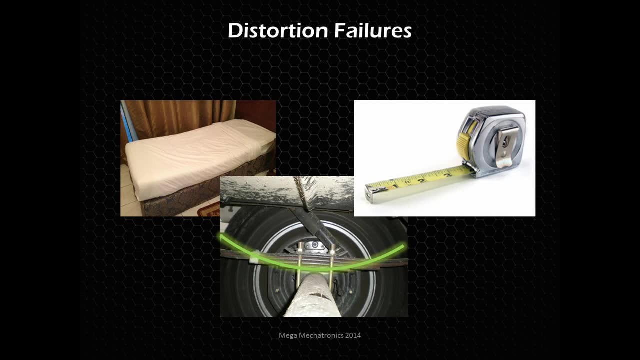 used to have a nice curve in it and now it's sagging and the car is sitting. funny, And even a measuring tape has this unique concave shape to that tape, So you can extend the tape out several feet. However, if you distort that concave, 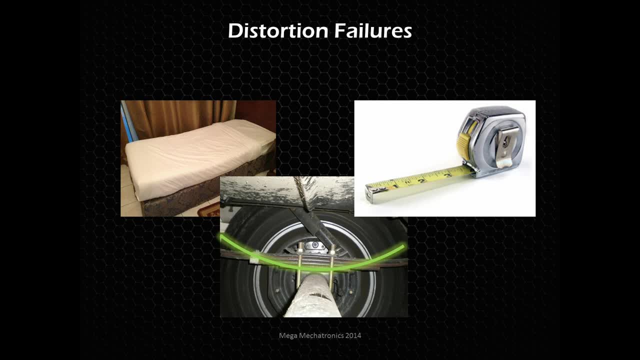 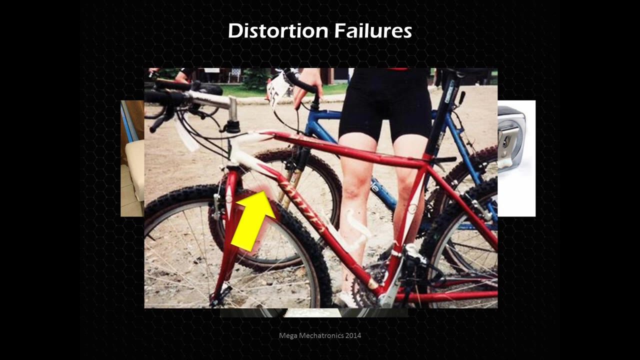 shape, it'll fail. It'll bend over and bend down. We can consider that a failure. Just because it got a little distorted it failed. And here's an example of a bicycle. The bicycle technically didn't break, but it did fail because it bent and changed all the. 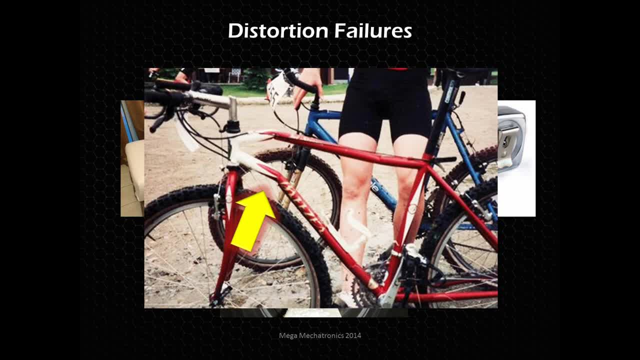 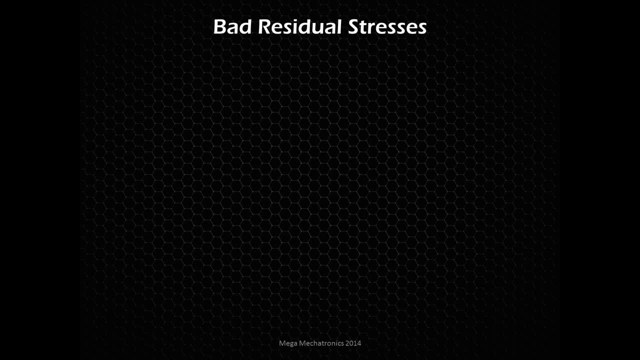 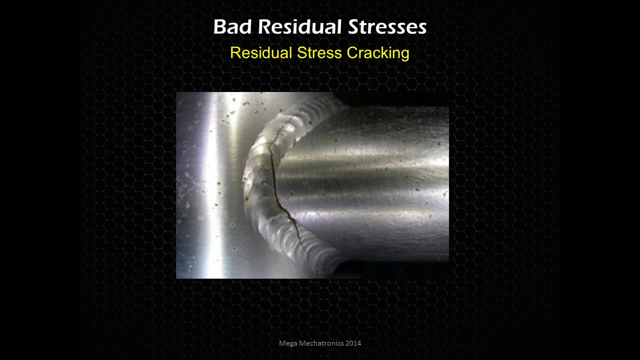 geometry and will probably eventually lead to a fracture failure. Let's look at some bad residual stresses. We are going to talk about residual stresses up here, but here's an example right now: Stress cracking. So these two tubes were welded together and they used the wrong manufacturing methods, or didn't. 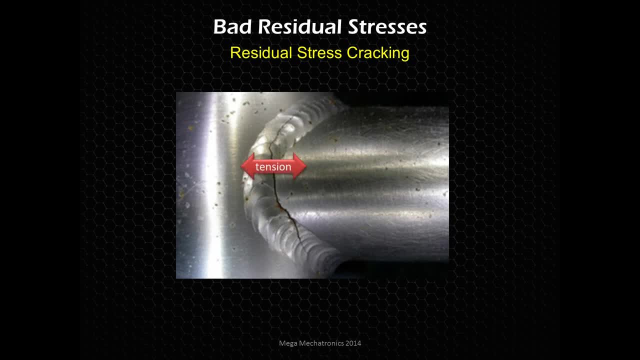 complete the manufacturing methods which led to a tensile force between these two different parts that are, after they welded and cooled it down. they're pulling apart. So having that residual stress in there and you can imagine a tiniest corrosion pit gets generated right at the 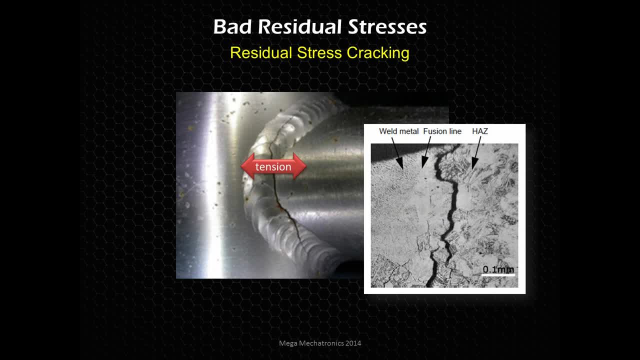 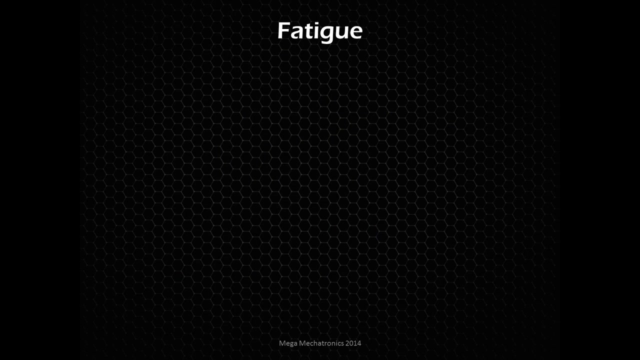 fusion line, that area, and then it just gets worse from there and cracks where a part that was properly manufactured could be filled with corrosion and, because it doesn't have these residual stresses in there, could maintain its structure. Alright, let's get into fatigue. 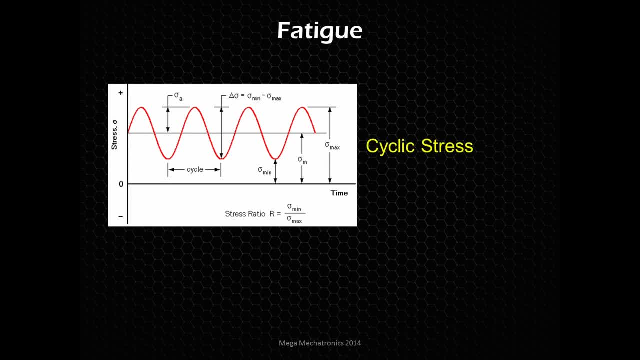 So fatigue is typically a cyclic stress on that part, So it's being constantly stressed back and forth. So, looking at this chart, you see two scales here: Stress scale on the vertical side versus time, And it's almost looking like, almost looks like. 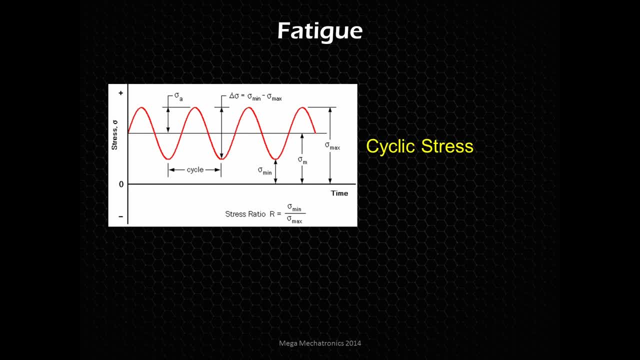 you're looking at a sine wave, Like the power coming into your house or electronics, But this is actually a stress. So in this particular example, very nice, even stress, and you see it's being stressed on the tension side. So the space between the zero and the minimum. 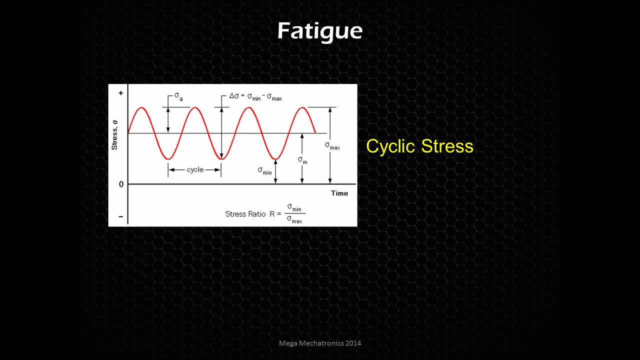 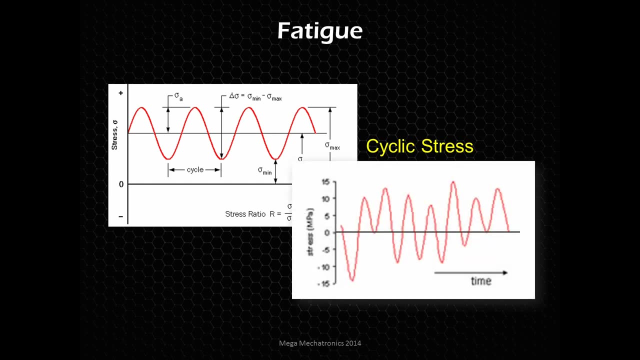 of those valleys is a pre-tension Because it's not reaching zero or it's not going into compression. So here it's just being stressed more and then stressed a little less on the tension side, And here's probably more real world stress when things are out of whack and it's not perfect and it's going into. 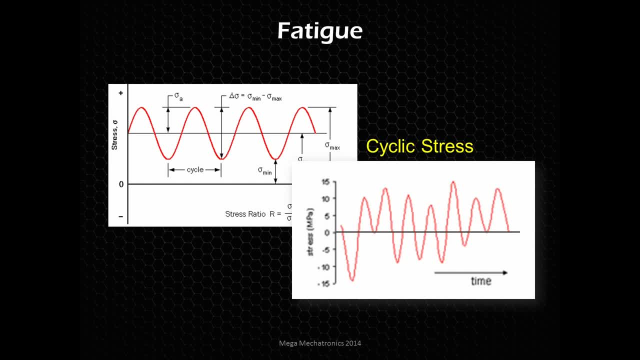 negative stress and the compression and moving around And things like this are curve balls. you can say Where some parts may enter a certain harmonic frequency, a natural frequency, and that stress being applied to that part matches that natural frequency. and then things get really excited, Things get out of control. 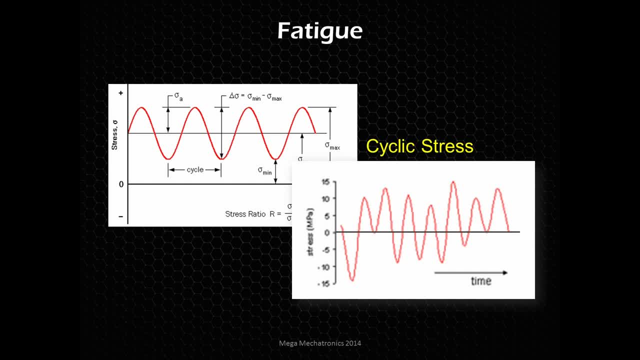 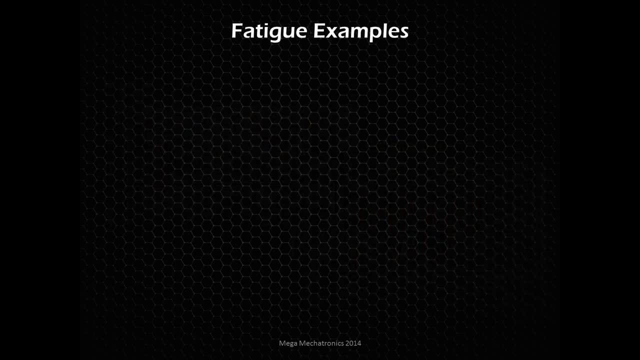 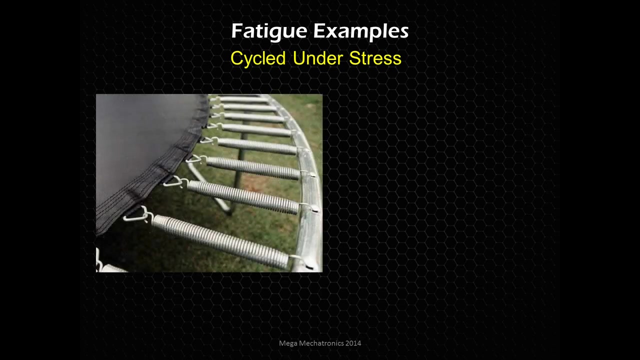 beyond what the engineers have expected, Or it just could be the nature of how that part is stressed. So some examples: Parts and objects cycled under stress. We have a trampoline And these springs. Well, we can see there's a little air. 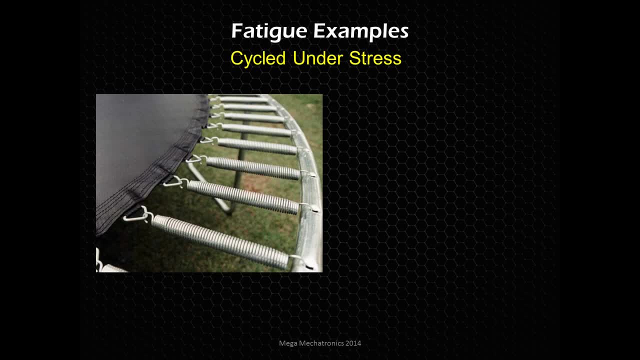 between those coils so we can say it's under a pre-tension. And then every time you jump on it it's going to increase the stress in those coils And if you put more people on it, or adults for say, they're going to reach a higher peak stress. 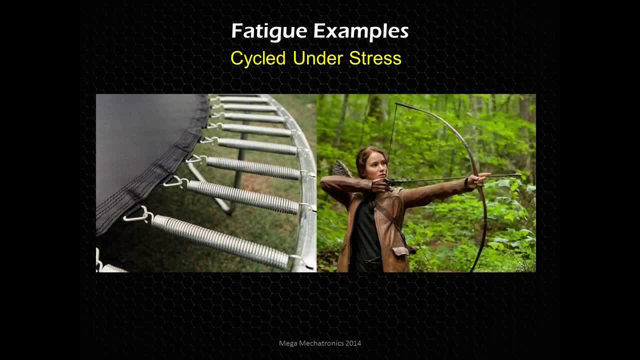 But they are going to be cycled every time you jump on it And the bow and arrow, So the bow is going to experience a cyclic stress. So every time you draw the bow it's going to increase the stress And then when you 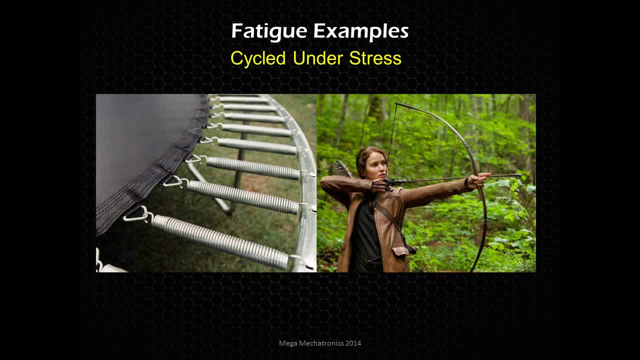 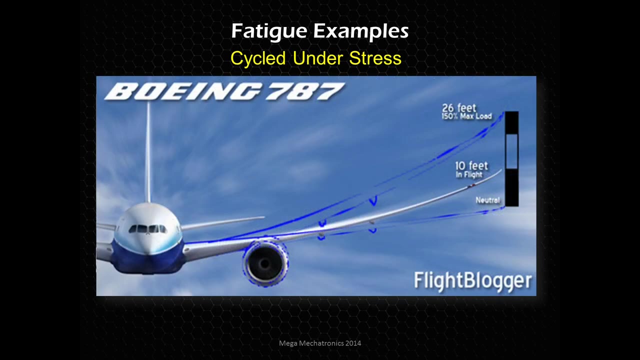 release the arrow, it's going to see an odd stress pattern and things like that. So bows, especially a wood bow, is not going to last forever because it's being cycled. And here's another fun example: The next time you're flying on a passenger jet and you have a window seat and you can see: 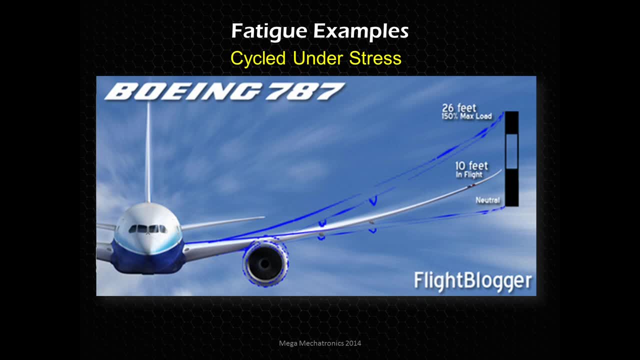 the wing Right before takeoff. reference that tip of the wing, Just stare at it. Reference the tip of the wing And as you accelerate up to speed you'll see that wing tip just lift And it's amazing and kind of unexpected. 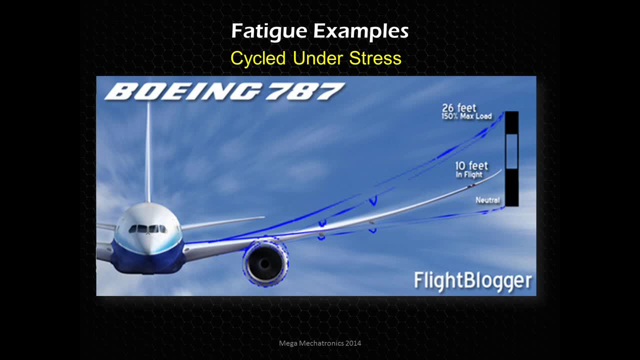 or a little bit scary, But that's how the airplane was designed And it's designed to handle these cyclic stresses, So don't be worried about it. There's very rare for an airplane wing to fail like that, But we don't want to forget there's thermomechanical. 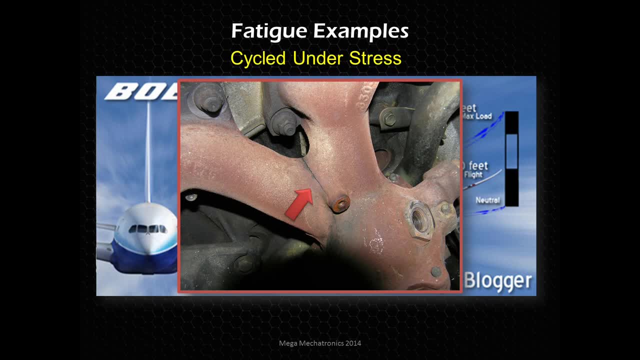 stresses, Because materials will expand and contract depending on the temperature. So here is a cast iron exhaust manifold on a car And you see, it developed a crack right here from just being every time, thousands and thousands of times, that this vehicle was cooled down and heated up and cooled down And that eventually, 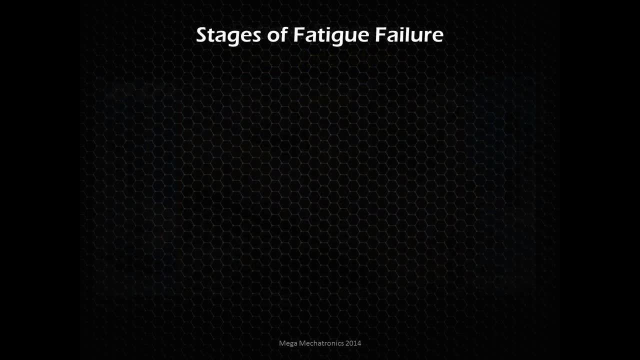 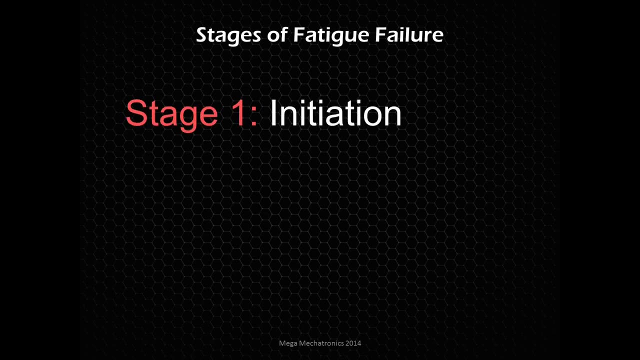 led to a fracture. So let's look at the stages, the official stages of fatigue failures. Stage one: we have the initiation. This is where it all begins And likely at a stress concentrator, But this is where the part starts fracturing. 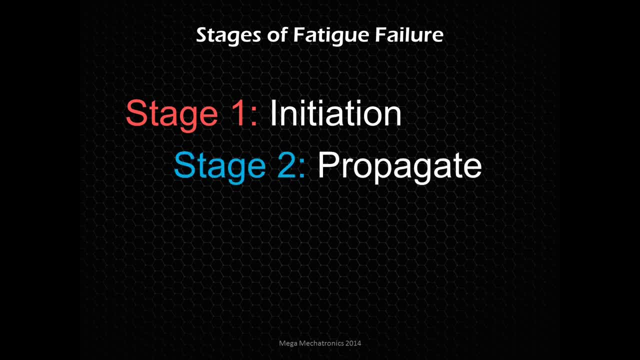 And then stage two is the propagation, Where that fracture. every time it gets loaded it starts growing, and growing in the very tiny microns, Very, very small amount. But depending on the material and the size of the load, it could take three cycles or it could take. 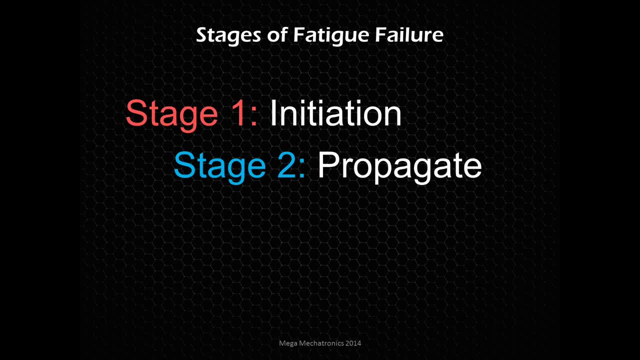 50,000 cycles, But every time you're loading that, that crack's getting bigger and bigger And that's the propagation stage, And then the spectacular ending would be the rupture. when we get our catastrophic-like failure, complete failure, where the part breaks, or 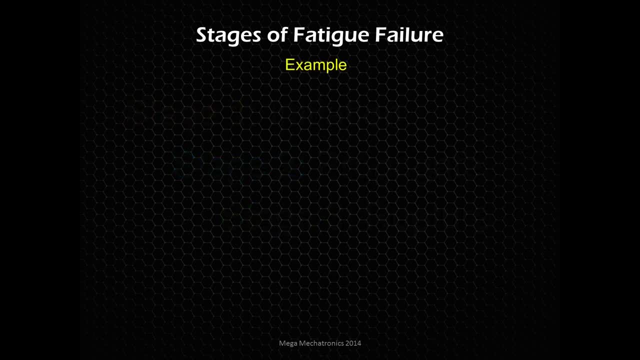 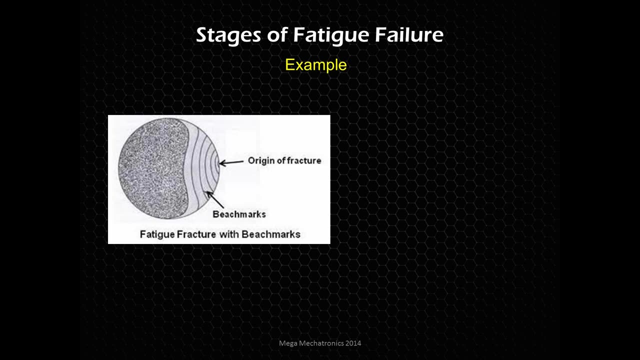 bends or collapses. So, looking at an example, we have a fatigue fracture with visible beach marks. There are beach marks that are typically visible to the eye And you can see how those beach marks radiate from the origin. So that's a very good indicator And this is the ideal. 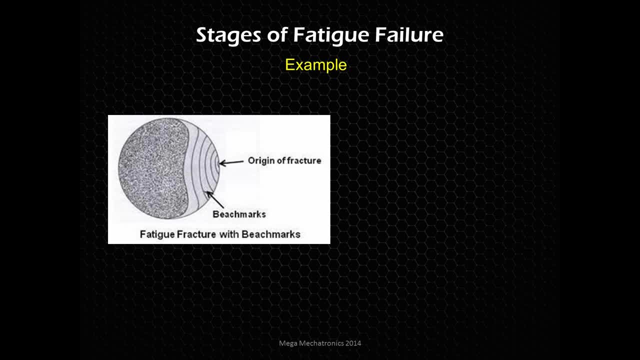 In the real world you don't always get so lucky to find these beach marks Or have actual access to an electron microscope to view the striations, which are similar to beach marks but appear in different materials and different sizes. So the striations are going to be much smaller And then you see that sort of 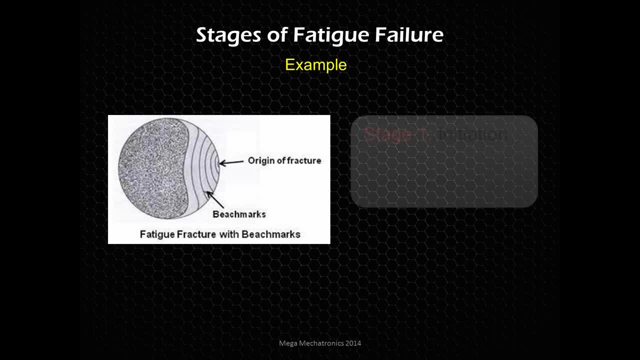 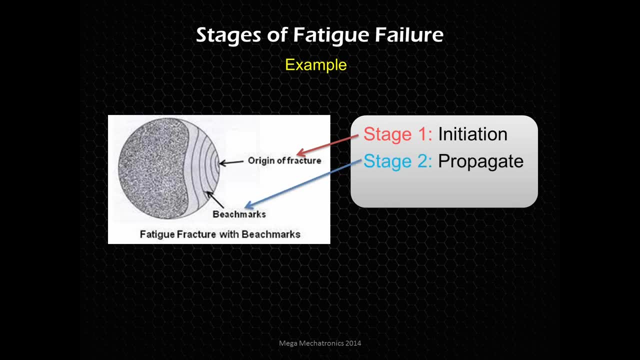 gray sandy area, and that's the rupture area. So we have our initiation at the origin, We have our propagation through these beach marks. So, starting from the origin, it's getting bigger and bigger and bigger until we reach the rupture stage where the part completely fails. 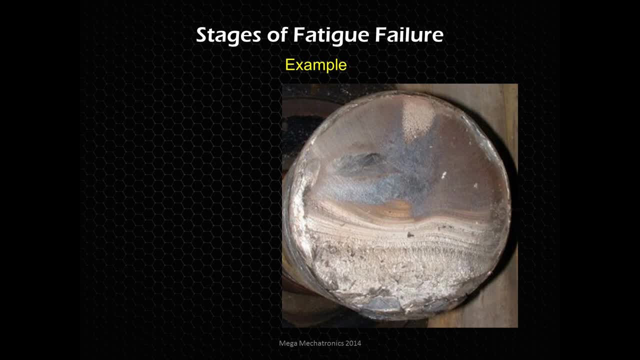 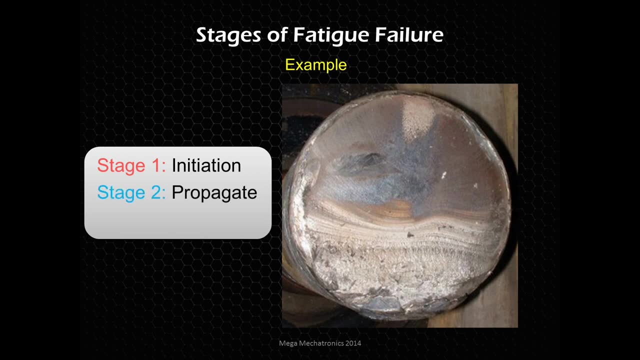 So let's look at a picture here And we can almost see if we follow the beach marks that we could visibly see in this picture. and we follow those beach marks, we can almost get a good idea where that origin was Around here. And then we're. 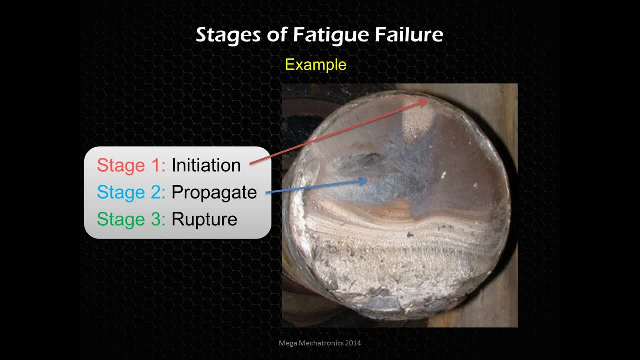 propagating over time And you could tell it was over time because there's rust. Look at that rust, that oxidized orange, dark brown surface. You can almost tell that this has been propagating for a while. And then it gets lighter and lighter until we rupture down here. 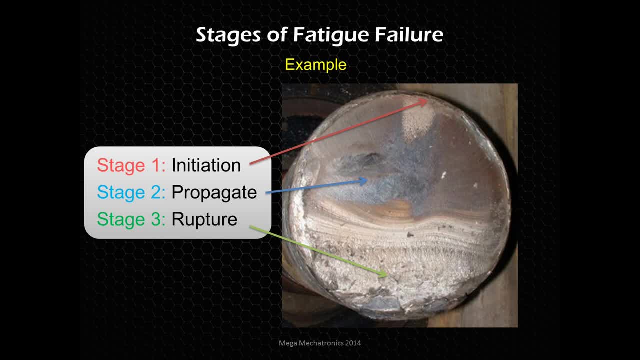 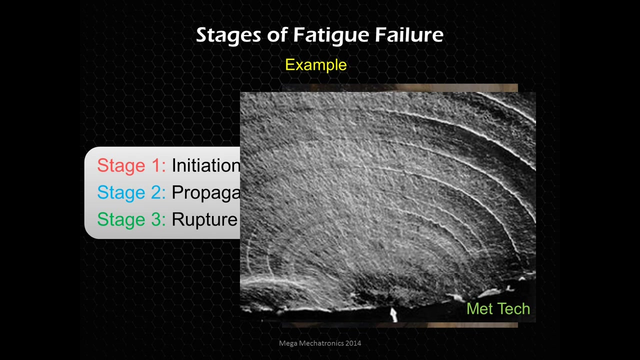 where we see sort of a brittle fracture And we can make out how far those beach marks made it to that final point. So it almost went through three quarters of this shaft before it finally failed. And here's a close-up of striations on a failed part, And you see, oh, this is absolutely beautiful. 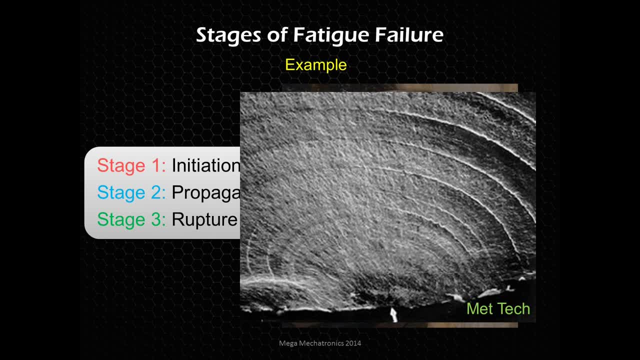 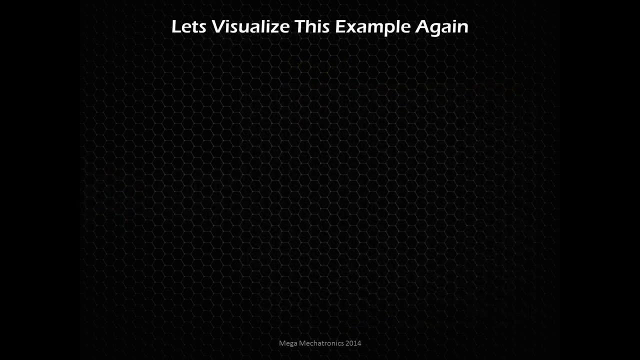 This clamshell, look And you see how it perfectly radiates. There's that little white arrow at the bottom, at the initiation point, at the point of origin, And you see how those striations just radiate out from there. So let's look at this example again. 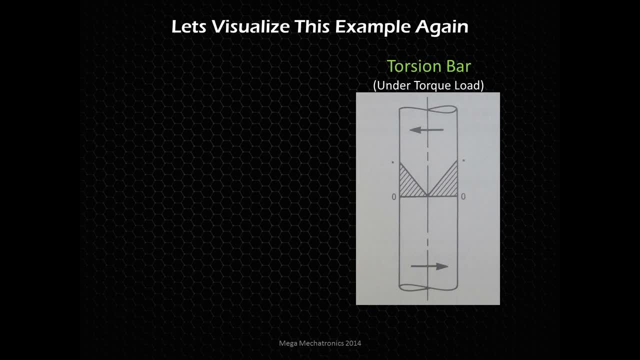 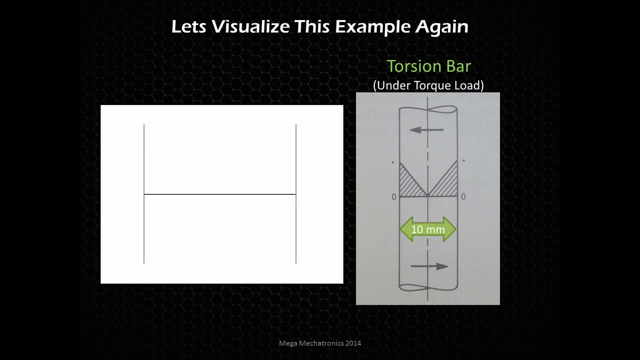 We have a torsion bar. It's under a torsion load, a torque load, And let's say this part is 10 millimeters in diameter. Let's put this into a graph form Just in case you're confused about the physical layout and the part being in the. 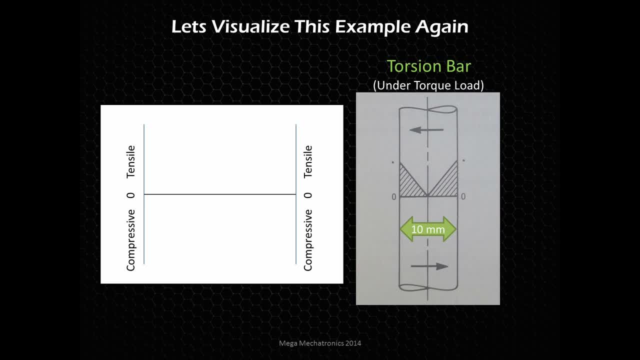 picture. So I'm going to draw the same exact graph over here. So we have our compressive zero point and tensile stress scales on the side. We have the depth. Now look at this depth. We have 10 millimeters here And you can see on the vertical. 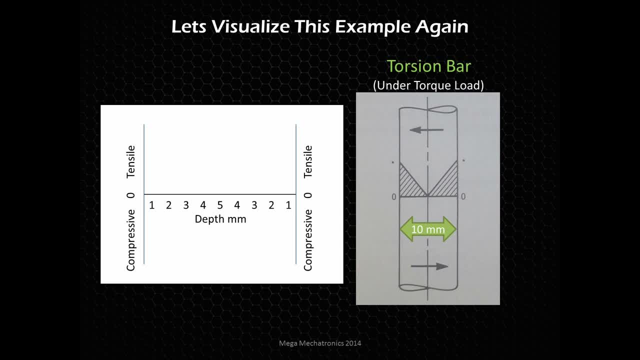 lines on each side. that's the zero point, Because those are the edges of the part, And as we move towards the center of the part, the depth goes to 5 and then it starts back to 4, because it's only 4 millimeters deep from the other line. 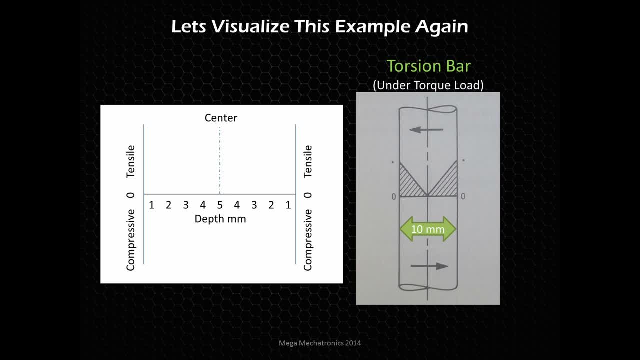 So here's the center of the part, This 10 millimeter diameter part, And here's the center point at the 5. And then, drawing the stress data, we can see it's on the tensile side And here at the very edge, at 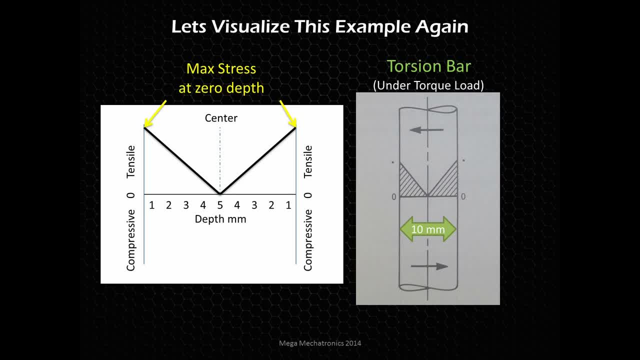 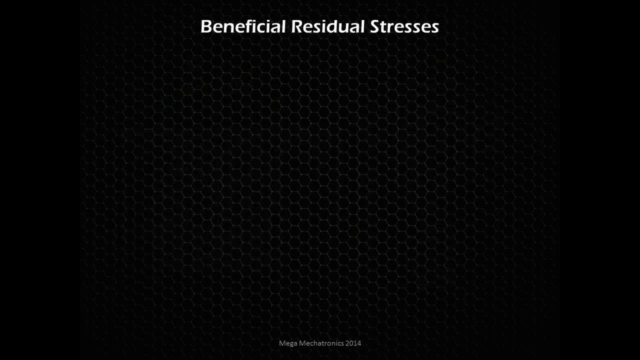 zero depth on the surface is the point of maximum stress. Now this is sort of a precursor to looking at this case study of beneficial residual stresses to prevent failure, Whether it's a distortion failure- what we're going to look at- or a fatigue failure, 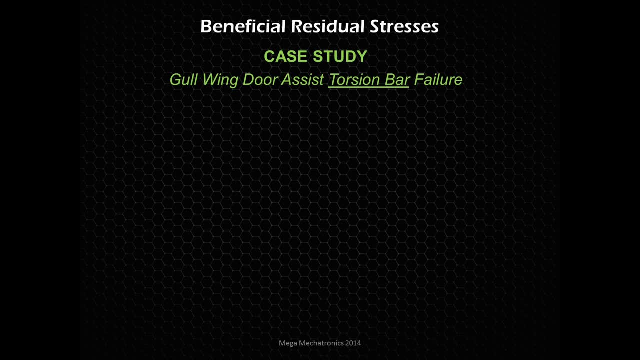 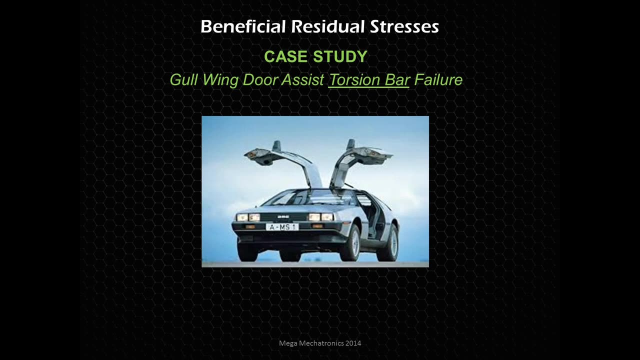 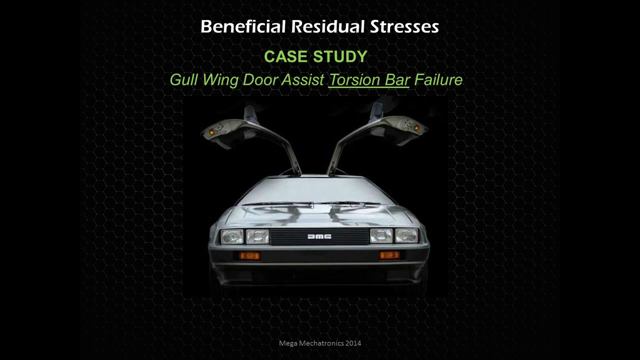 So let's do a case study on the gullwing door assist torsion bar for a DeLorean, the back to the future car. There's actually torsion spring bars that assist the opening of the door. So looking from the front, the doors are fully open. But let's say 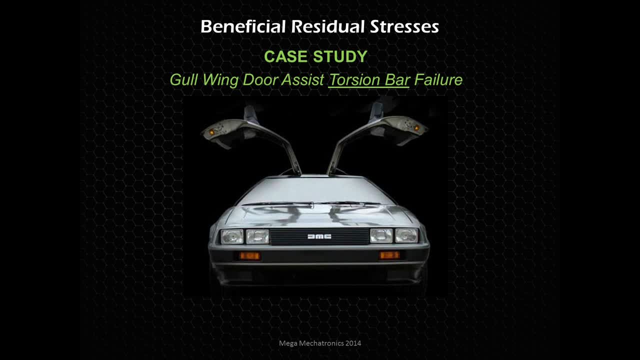 one of the cars got through the factory and after they closed the door and then opened it for the second time, they found that the door on the passenger side was sagging for some reason, And that, of course, is a failure in quality, Definitely a failure. 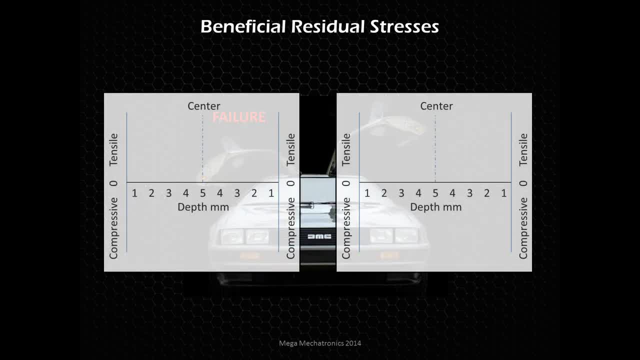 So let's look at what happened here. So we have our passenger door torsion bar and we have our driver door torsion bar And let's say, the dashed orange line is the material limit, That's the, whatever material they're using, that's the. 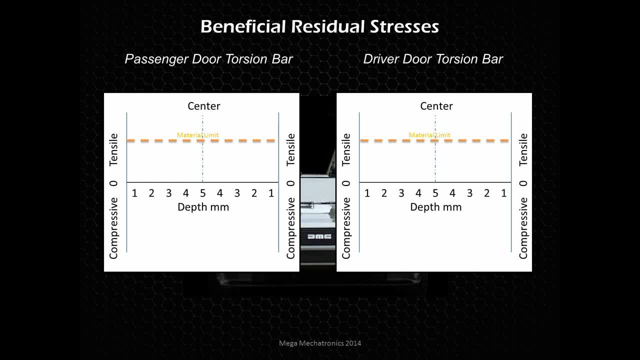 yield strength. for example, before it's, the torsion bar starts permanently getting deformed and failing. So let's say, the scientists or the quality engineers found out that there was no residual stress on the passenger door torsion bar And on the driver side. 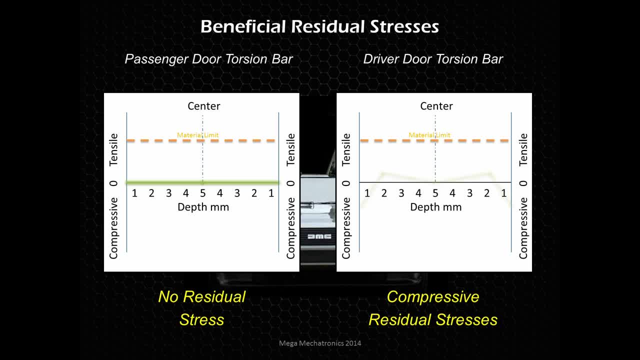 where it didn't fail. they found compressive residual stresses at the surface. So both of these parts are unloaded at this point. They pulled them out of the vehicle and they're just sitting there on the table. So you can see on the driver side. 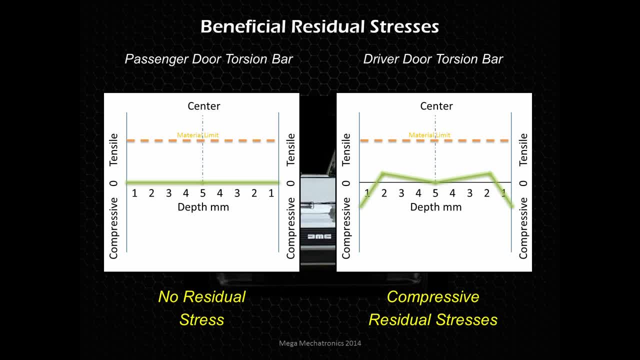 door. at the surface of the part there is a compressive stress And then, as you go deeper it'll transition into a tension stress, because these stresses have to balance out within that material. But you see, there is a compressive residual stress at the surface. 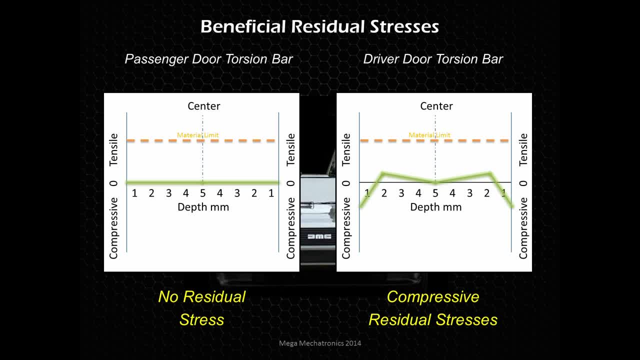 of this torsion bar. So what happened? Why did it fail and why was that sagging? Well, when they closed the door for the first time, the material stressed beyond the stress, surpassed the material limit, the limits of that material, and caused a plastic. 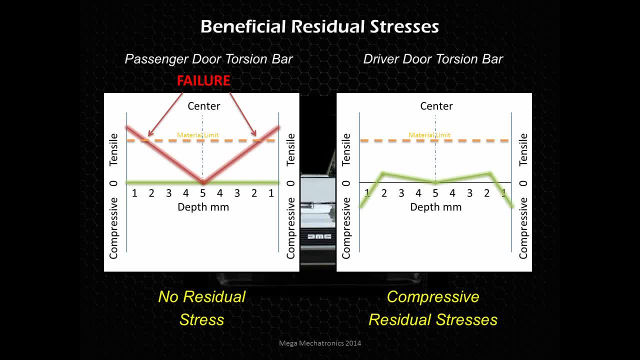 deformation which changed how that torsion bar works and it actually loses its strength. So why did the driver door survive? Well, when they closed the door and you see those little spider legs, you could see how, on the very edge, where the compressive residual 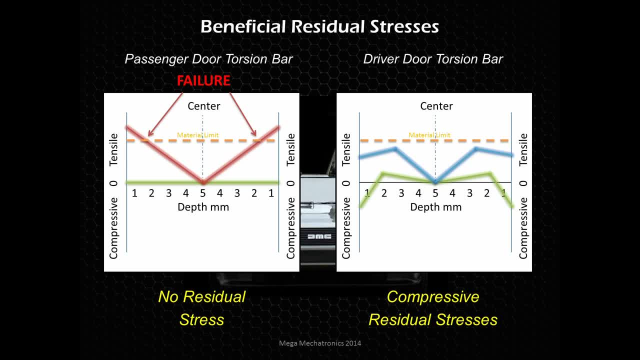 stress was how it compensated for that and how it prevented it from, at the surface, exceeding the material limits. Look at that. So, going back and forth, you could see how that compressive residual stress reduces the maximum tensile stress on the surface of the part for the same exact. 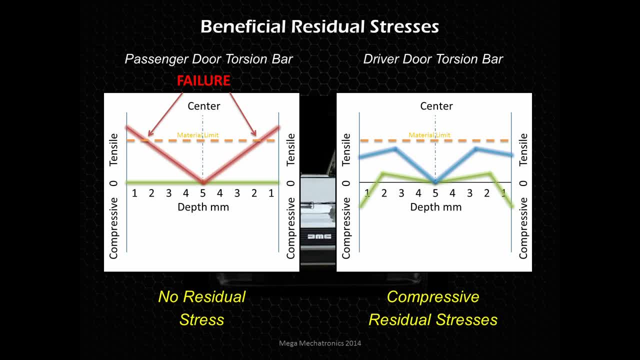 load. So this concept here is what makes valve springs so durable and makes them last so long. Crank shafts and any parts that are cyclically loaded Aircraft- This is a very big deal, These compressive residual stresses within airplane parts. 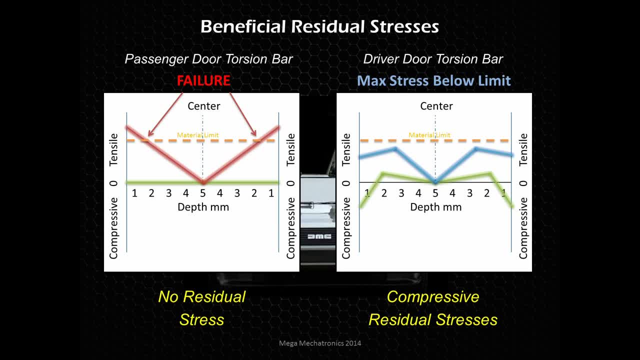 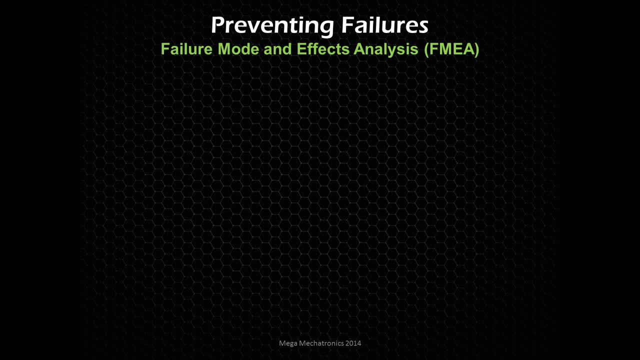 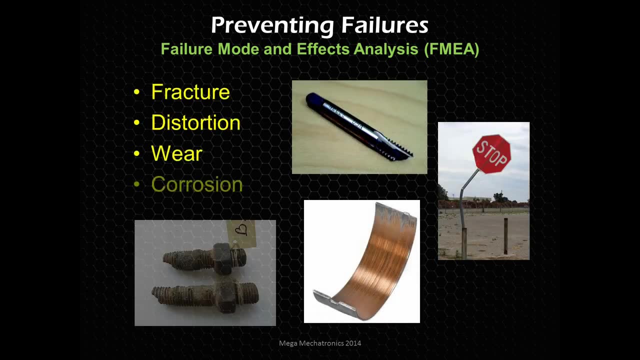 Very important. So, again, the max stress is below the limit. So, preventing failures, Failure mode and effects analysis: Well, you need to look at your part- and for fractures. So why did it fracture? Well, probably because it was fatigued, It was overstressed. 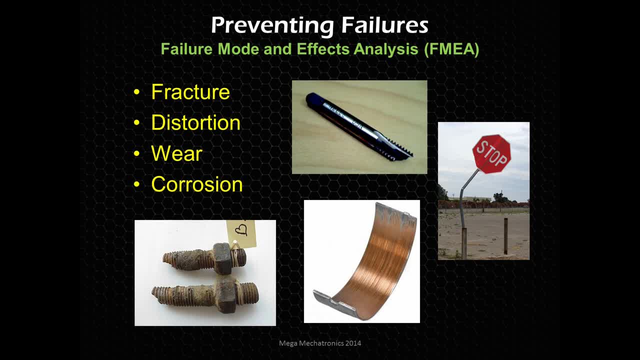 There was corrosion. So things you can change for distortion failure is prevent that distortion. Prevent something from hitting it. Prevent a car from running into it. Increase the structural rigidity of that system. Where Do you need to improve the lubrication systems? 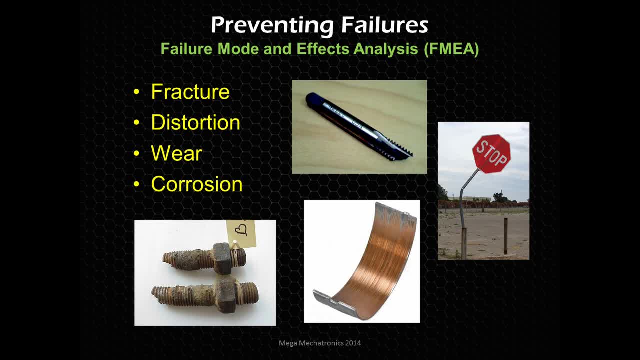 Did you forget to lubricate it? Does it need a different type of material that are mating with each other? Does it need more surface area? Things like that. And corrosion. What happened there? Was there galvanic corrosion? Were there dissimilar metals? 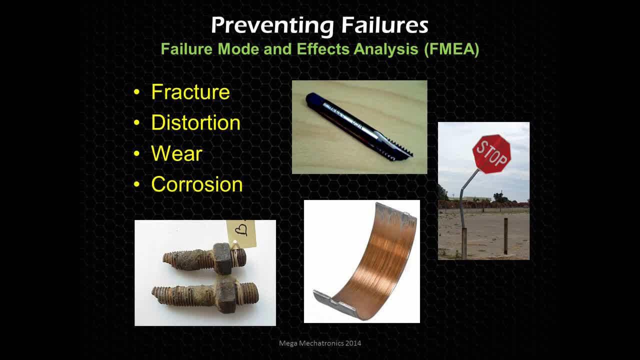 Did the paint chip off? Did you not paint it? What type of environment Was it designed for? fresh water but was brought to salt water And things like that. So you need to find that root cause. Why did it fail? Why did it wear? It broke, but it broke because of this and this.